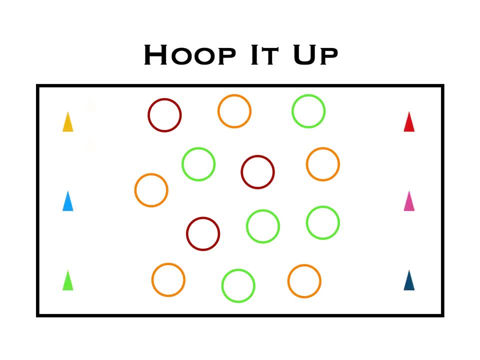 And you're going to place down cones, one for each team that you have. In this example, we have six teams and each team is a pair of students And they're going to start off at their cone and you're going to give each pair of students a pair of skipping ropes.